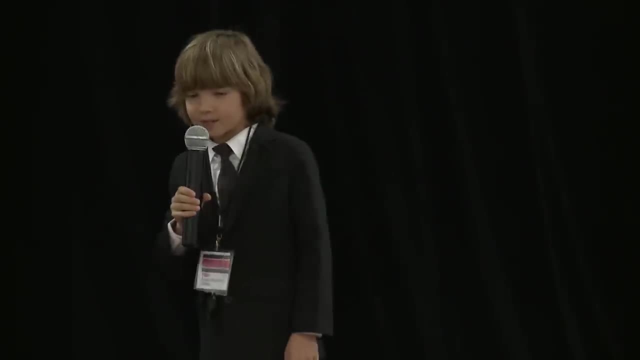 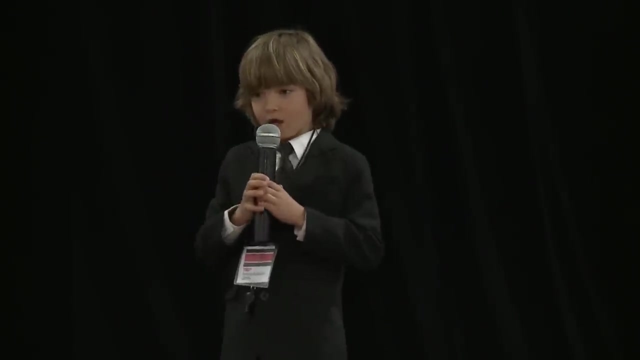 and less fidgety on days when they had recess. Stress impacts on learning and health. For many children, especially those considered hyperactive, recess is an opportunity to expend energy in a healthy, suitable manner. Recess develops social skills. Recess may be the only time of the. 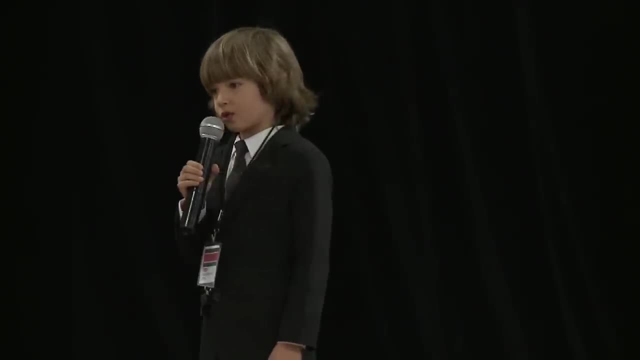 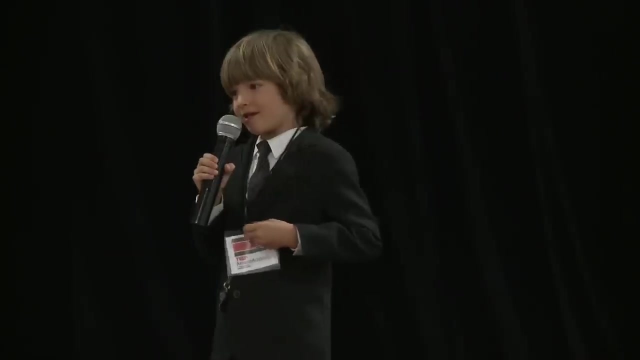 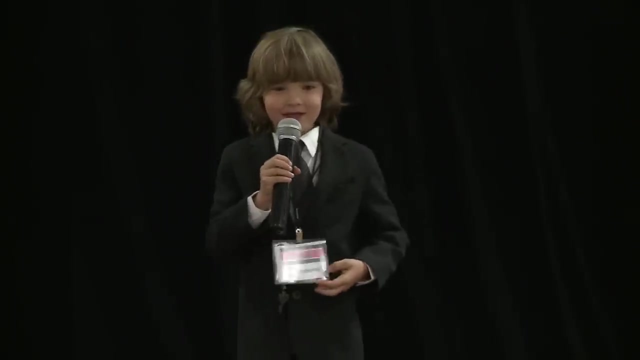 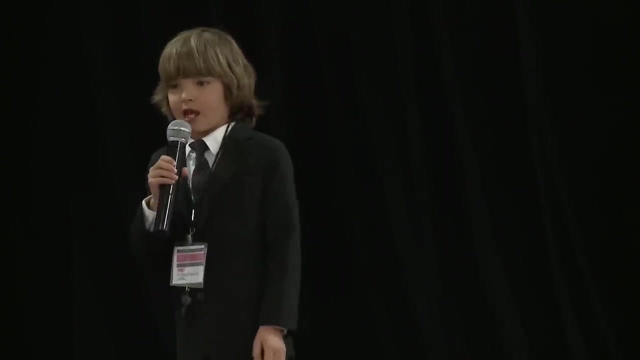 day when children have an opportunity to experience socialization and real communication. The outside light triggers the synthesis of vitamin D, which many studies have shown increases academic learning. The outdoors is the best place for children to burn calories, have healthy, healthy, harmonious and similar physical activity. Recess is a way for children to 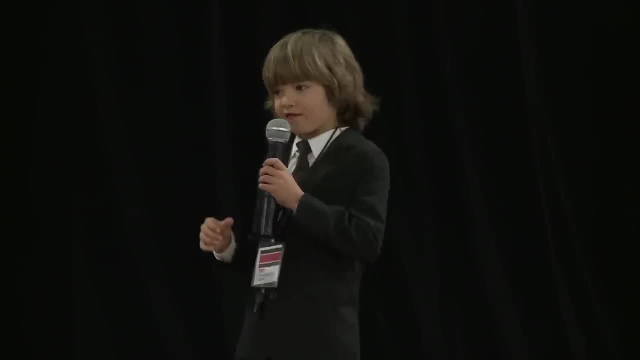 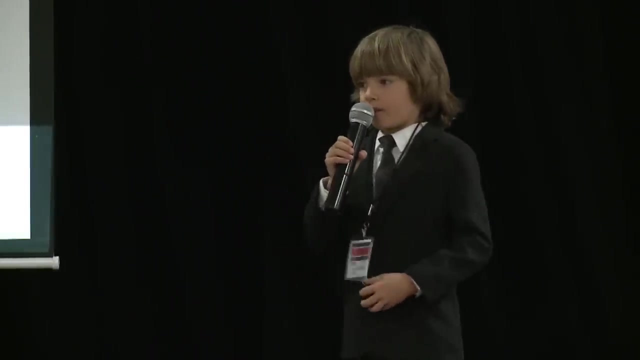 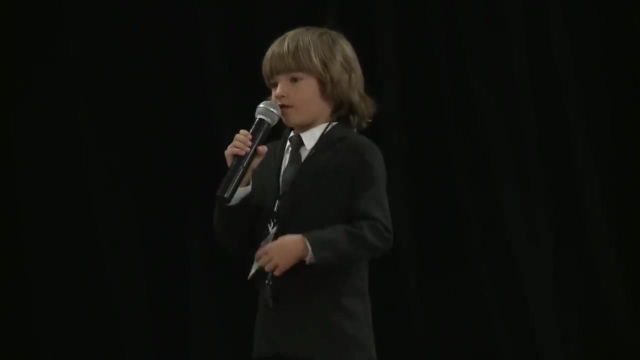 learn new and fun activities, to learn physical movements, to balance their mental and physical skills and to experience the pure joy of movement. According to Ray Pica, who is a children's physical activity, specialist, recess may be the only time to have a break. This shows that 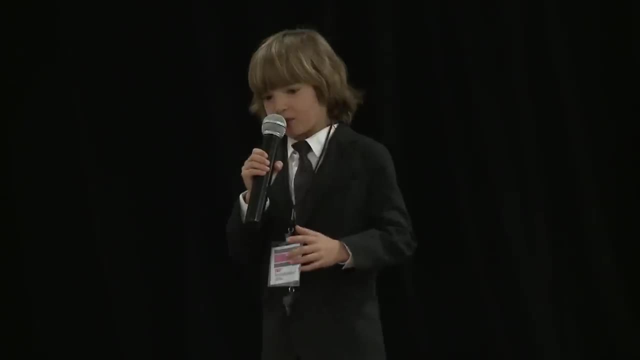 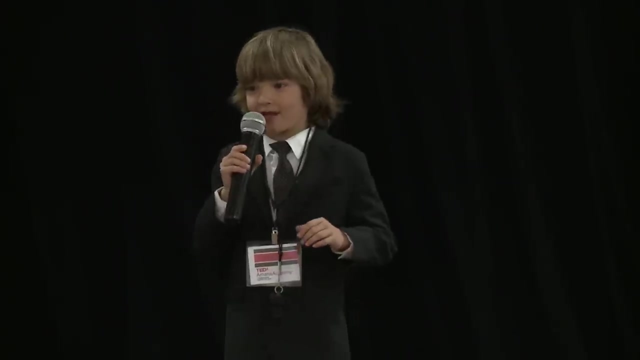 when you have physical activity at school, you usually have more physical activity at home, and children who have, who don't have the opportunity to be physically active during the school day, don't usually compensate during the after-school hours. Running around helps the brain. 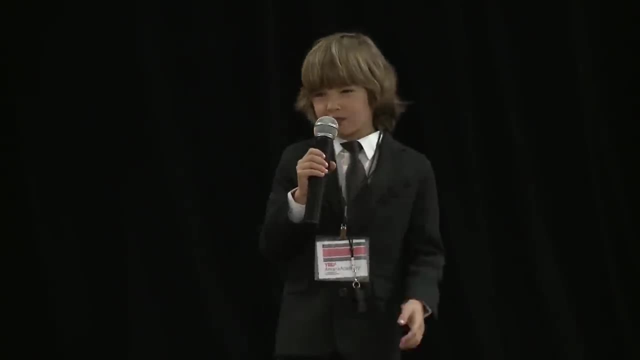 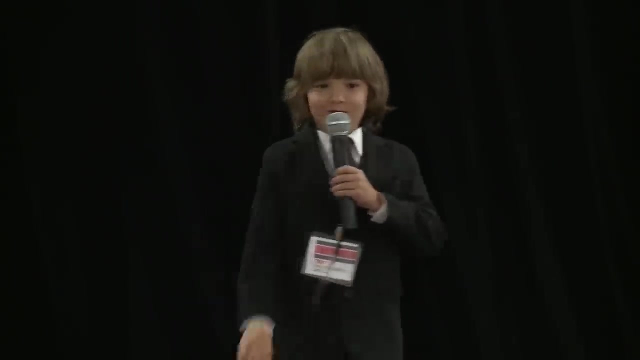 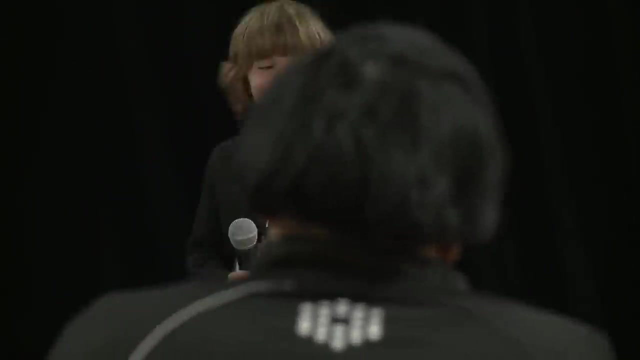 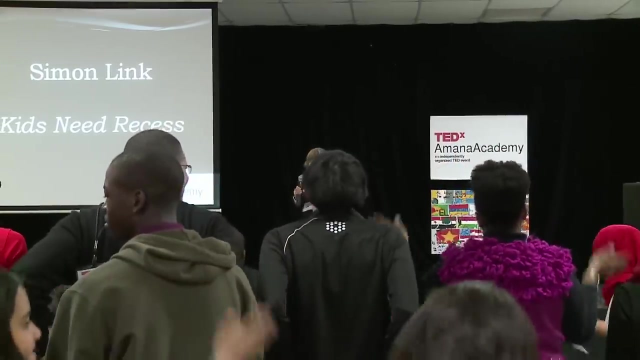 Thanks to advances in brain research, we know that most of the brain is activated during physical activity, much more so than being a couch potato. Now, stand up and do 10 jumping jacks when I say: go, Go, 1,, 2,, 3,, 4,, 5,, 6,, 7,, 8,, 9,, 10.. 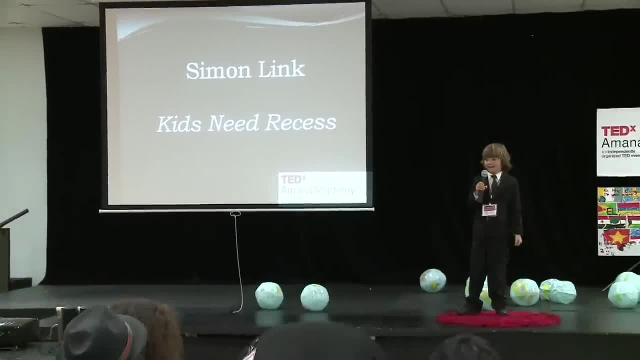 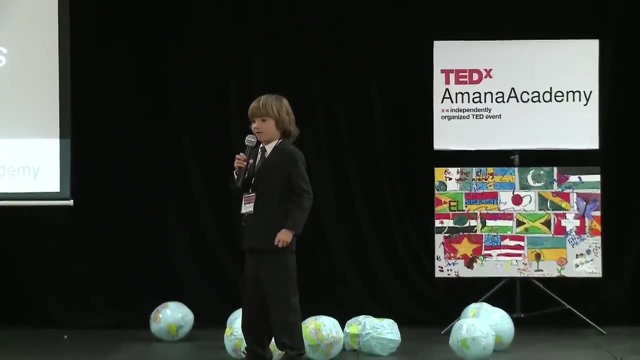 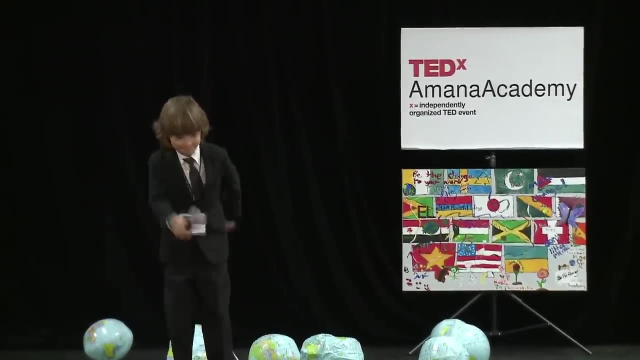 Now sit down. I imagine a world where every child gets lots of playtime. I hope that if you have children, you will make sure that those children get lots of playtime. Thank you, applause.